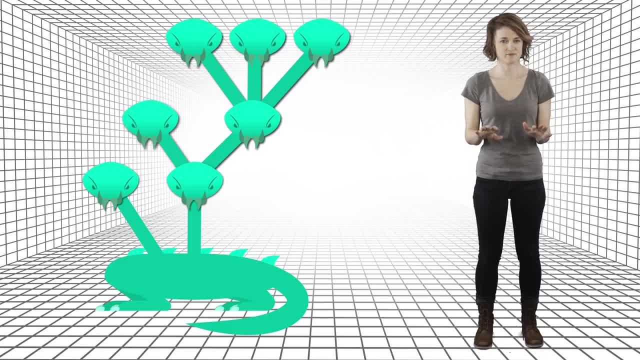 For the sake of example, I'll just try to defeat this Hydra. For the first move, I'll chop off this head, the one attached to the body. In that case, nothing happens, Nothing regrows and the Hydra is one step closer to defeat. But these heads, the ones attached. 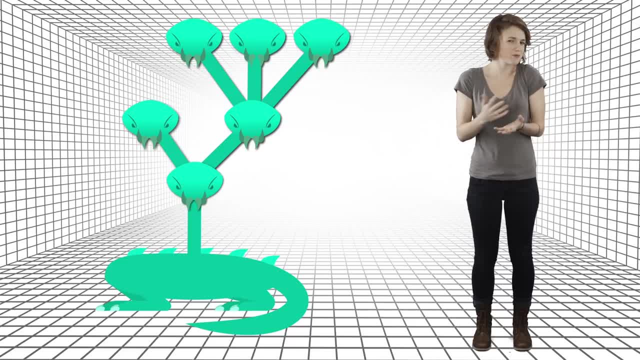 That might sound a bit complicated, but let's just see what happens in our example. What if I chop off this head, Go down the neck toward the body? For clarity's sake, we'll mark that edge in blue. Now the Hydra regrows two new copies of the blue edge. 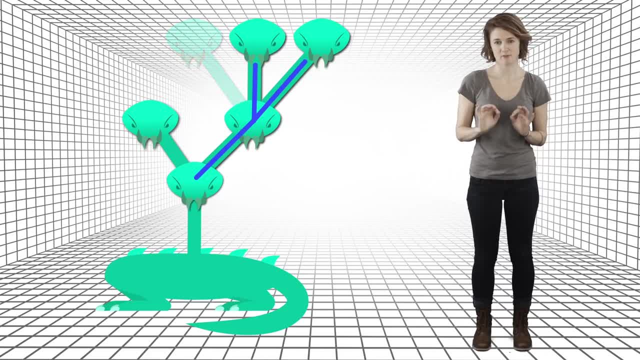 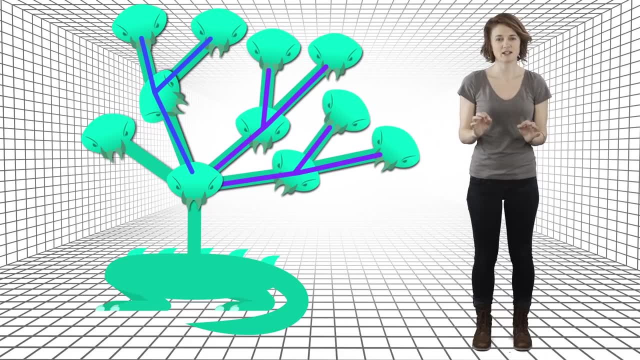 edge and everything above it except the heads we chopped off. The copies of the blue edge are temporarily marked in purple just to help show what's going on, But that didn't seem to help anything. The Hydra looks bigger Now there are 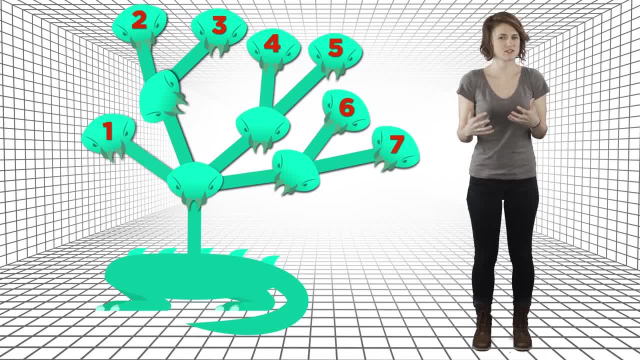 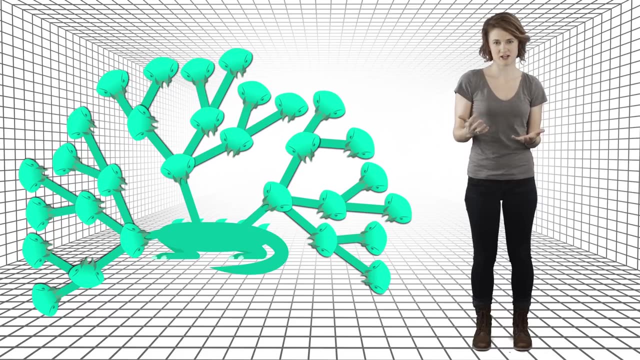 seven options for which head to chop off, so I'll choose this head Again. we go down one edge and mark it in blue. The Hydra generates two new copies of the blue edge and everything above it, so we get this. But that also might have been a. 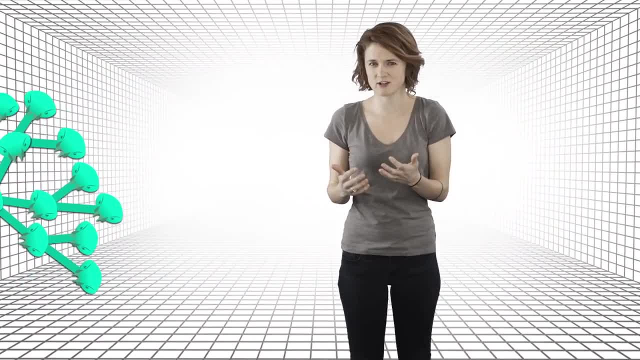 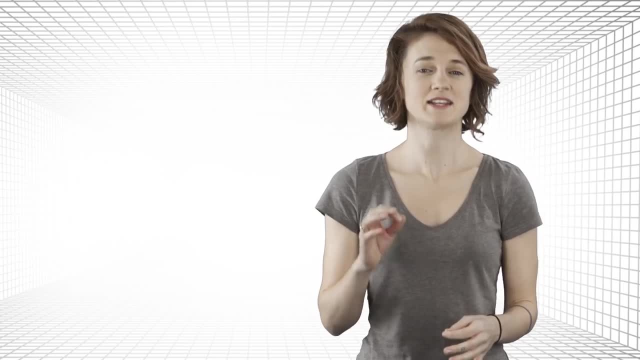 mistake. Maybe I'm just not doing it in the right order. Do you think it's possible to defeat the Hydra, And if so, can you come up with a better strategy? Now I'm going to start to answer these questions. It'll take a few steps At any. 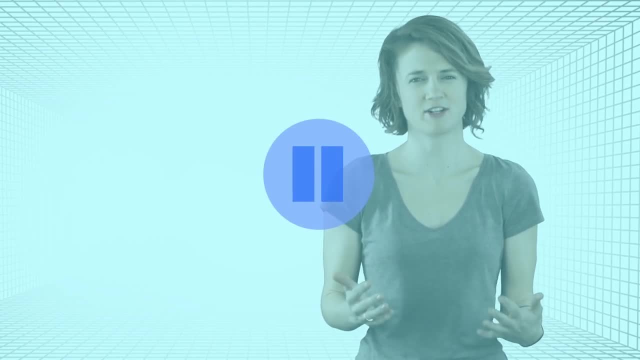 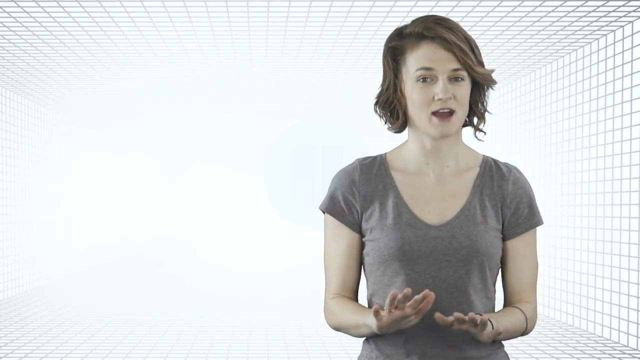 point. you should feel free to pause the video and think about it on your own. It might help clarify things, to draw some pictures and work out some stuff. So let's get started Now. here's the big theorem: No matter what order you, chop off the heads you. 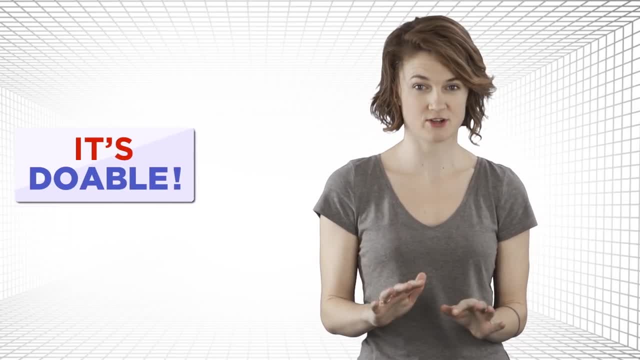 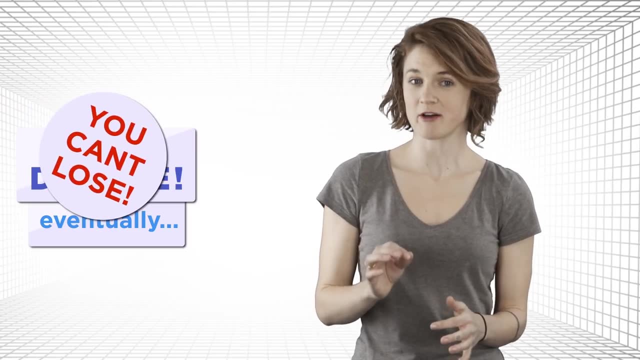 will, in a finite number of steps, defeat the Hydra. That is eventually- and that might be a really long eventually- you will chop off all the heads. This theorem can seem totally counterintuitive, given how quickly the Hydra appears to be. 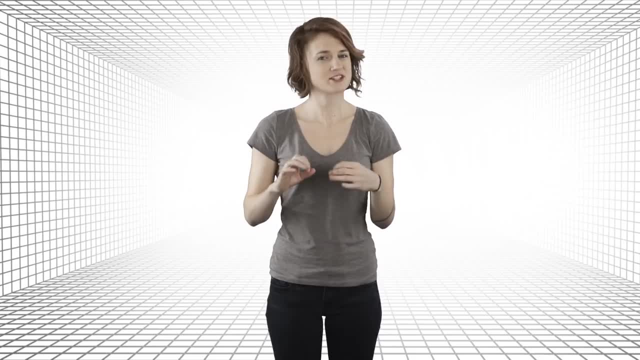 growing To begin to understand what's going on. let's try something very common. Let's say that we're chopping off the Hydra. Let's say that we're cutting off all the heads, But you're trying to pleased that Hydra. However, 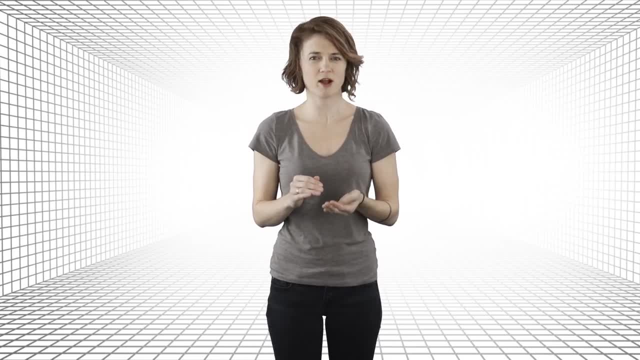 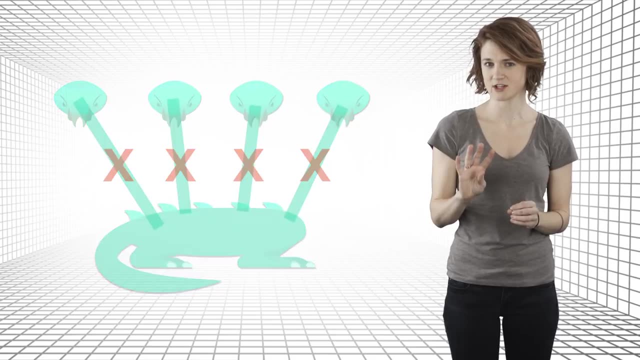 even so, when you look at the occurrence of switching heads, you get the same same viewpoint here. It's a simple example. to give a title, The être is common in mathematics. We'll look at examples of small or simple Hydra First. 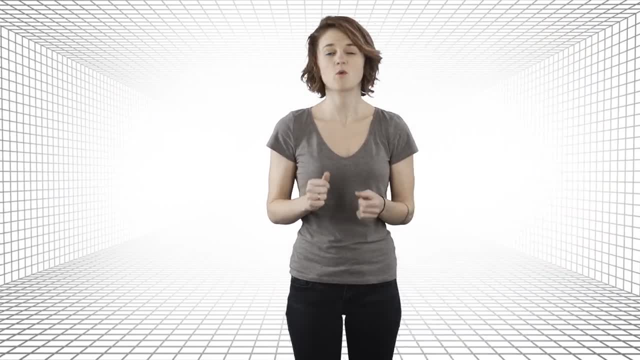 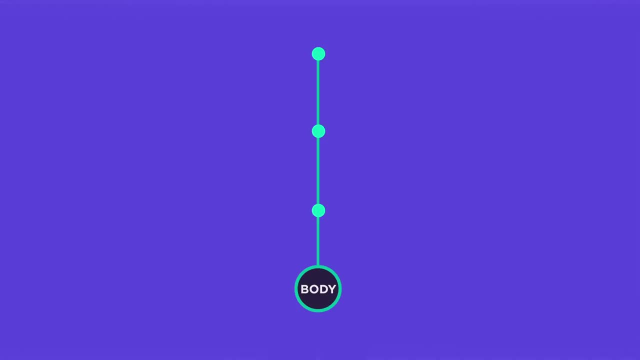 the simplest kind of Hydra is probably one where all the heads are attached directly to the body. If it has four heads, it takes four chops to defeat the Hydra, And 10 heads just takes 10 chops Easy. What if the Hydra's just a line as? 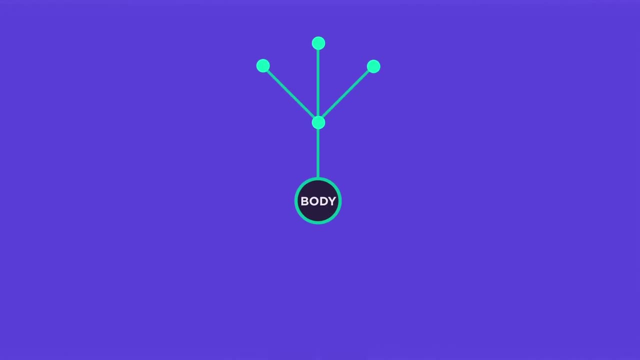 so we'll do that. Then there's not a whole lot of other options, so we'll just keep going. As we chop off the forking branches, they're replaced by equally long non-forking branches, until there are nine branches of length two Then we. 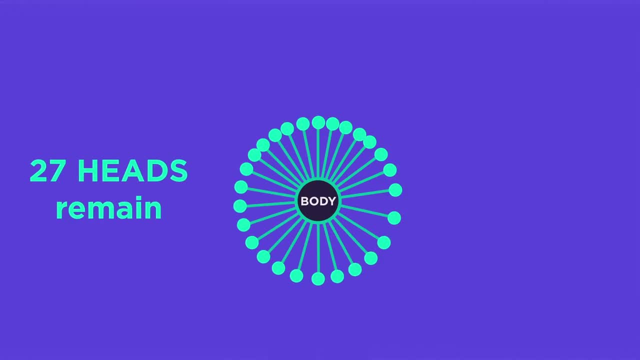 chop off the ends of these until there are 27 heads connected directly to the body. Finally, 27 chops later, we're done: Hydra defeated. Here's what the first 15 steps look like if you start with a hydra. that's a line of height, four After. 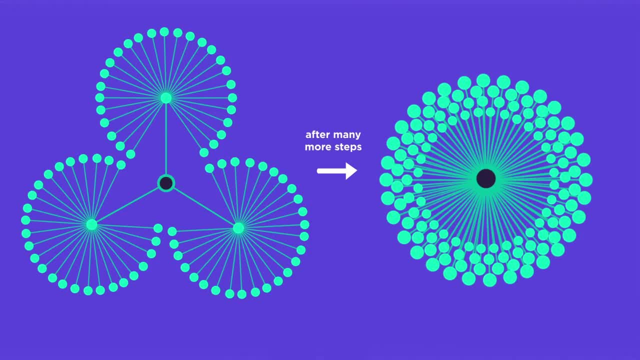 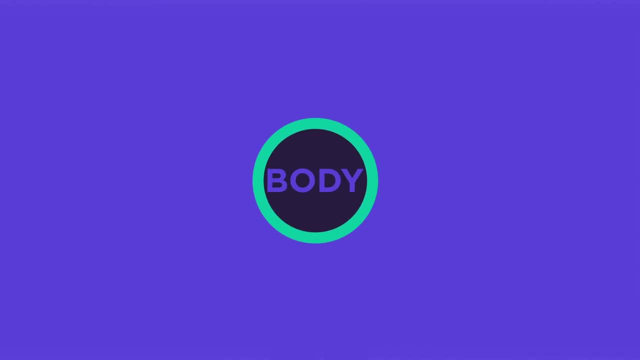 many more steps. this hydra will look like a spiky ball, just a body with many heads attached directly to it. Then you'll be able to chop off each of those heads and defeat it. Here's a challenge question: How many heads will be in this? 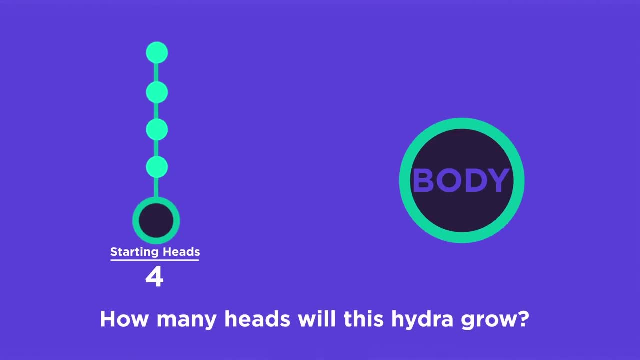 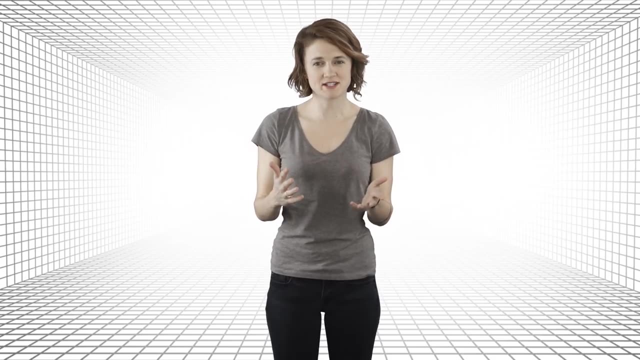 spiky ball if the original hydra is a line of height four, And how many steps will it take to finally defeat this hydra? Okay, after all that we're done, all those examples, what have we learned? First, notice that the hydra never becomes taller. 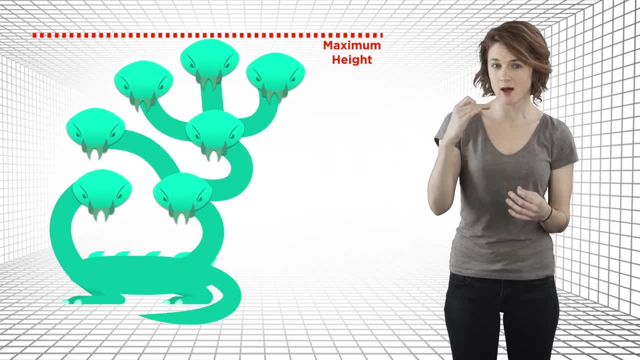 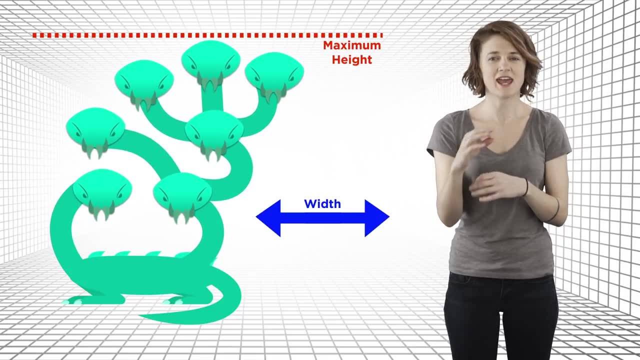 That is the maximum height of heads that are stacked on top of one another- never grows. The hydra's becoming wider but not taller. It's kind of detangling itself level by level until it just turns into a giant spiky ball. 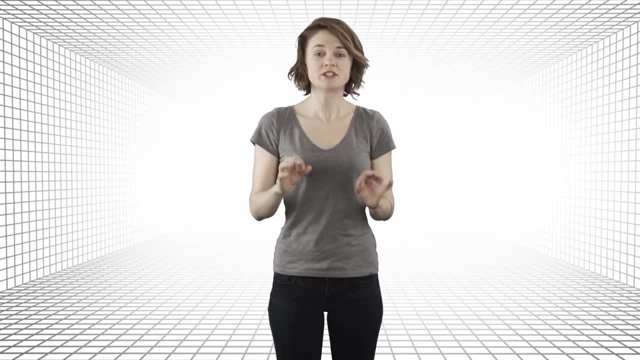 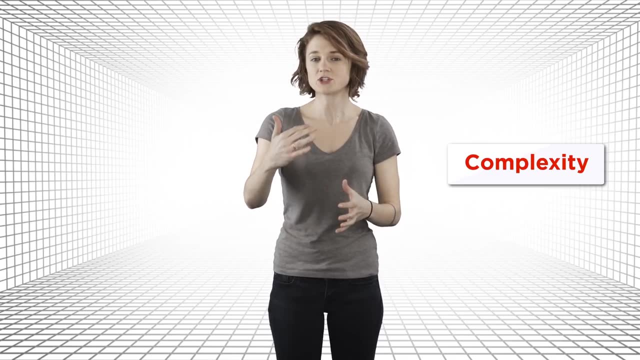 To prove this rigorously, like we do in mathematics, we'll need to encode the hydra's complexity To show that the hydra will be killed in a finite number of moves. we'll need to show that the hydra's complexity goes to zero. 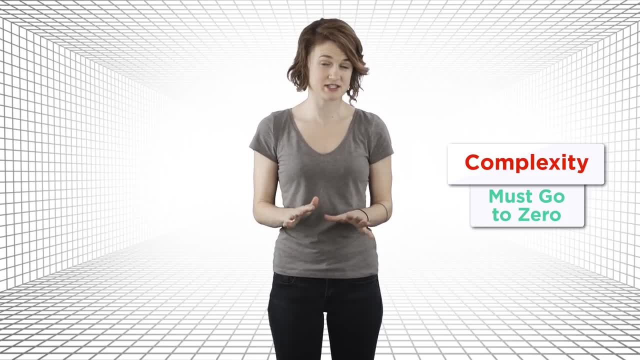 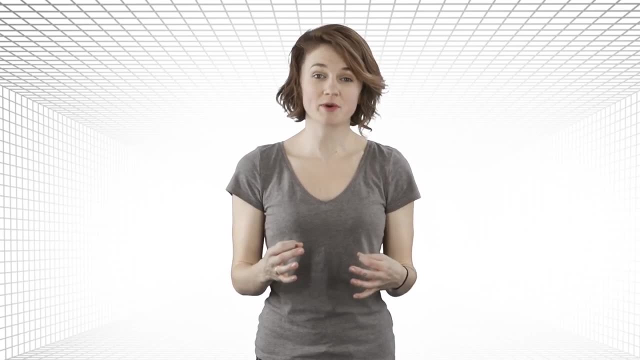 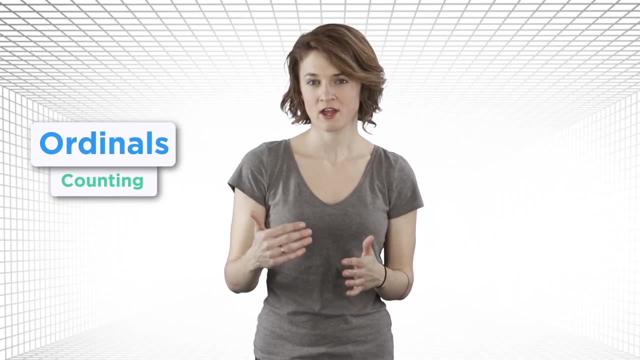 That is. we'll show that it eventually becomes the simplest hydra, a single body with no heads. Here's where it gets really weird. The tool we're going to use is ordinals. Here's a crash course in ordinals. Ordinals are the numbers we use to count. 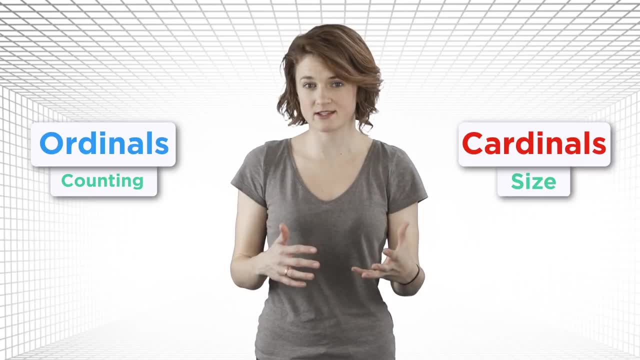 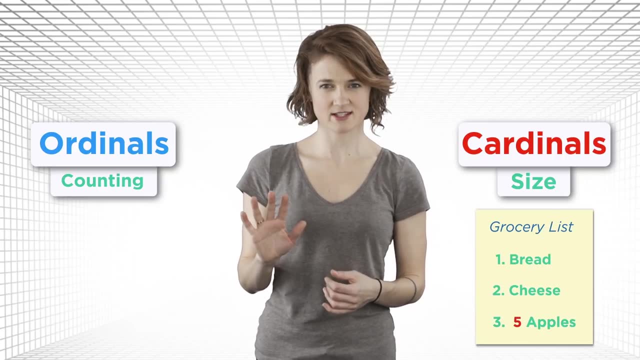 They're different than cardinals, which are the numbers we use to tell size. If five apples is the third item on your grocery list, the number five is a cardinal, It's about size, And the number three is an ordinal, It's about counting. 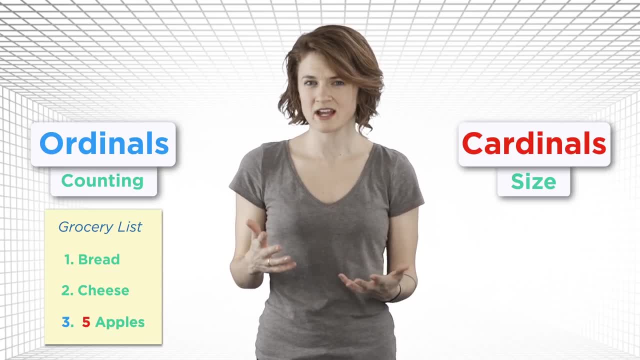 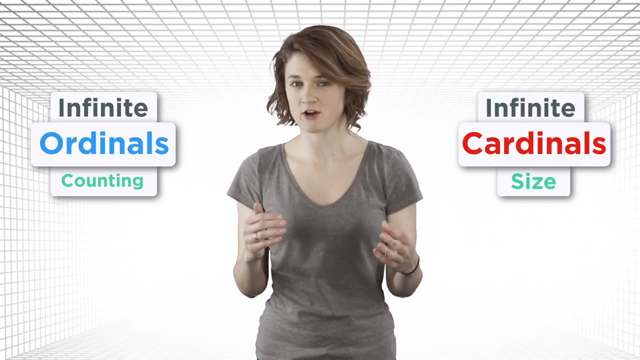 The reason they usually don't teach you about ordinals and cardinals in school is that there isn't really a difference if you're only talking about finite numbers, But infinite ordinals and infinite cardinals are different. Our episode: A Hierarchy of Infinities. 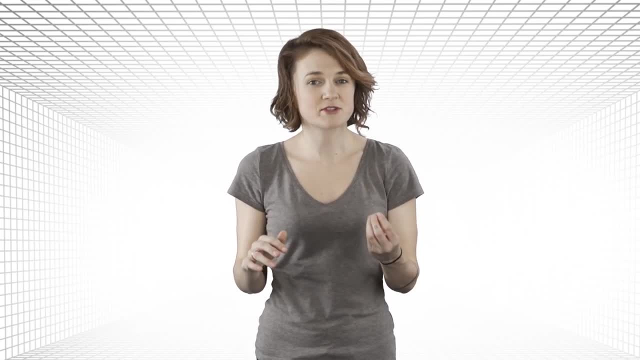 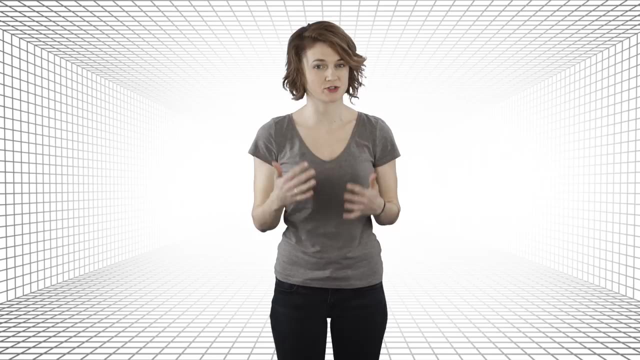 was about cardinals sizes of infinity. This episode is about Ordinals infinities to count with. I'm not going to go into a detailed explanation of how ordinals work. There's plenty of other resources for that. I'm just going to describe the part we need. 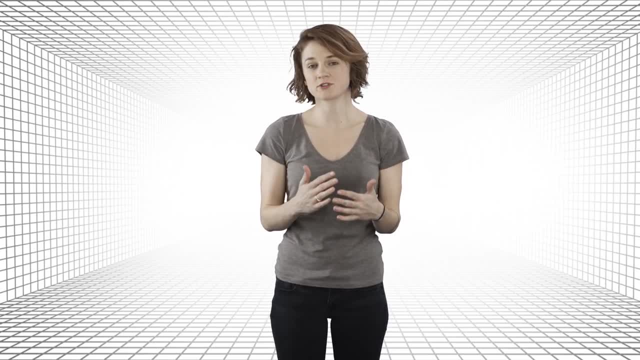 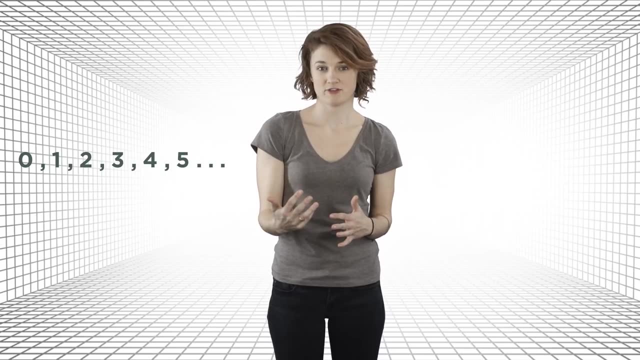 the ordering of the ordinals. The smallest ordinals are finite: 0,, 1,, 2,, 3,, 4,, 5, and so on. And then, after all that, comes omega, the first infinite ordinal. Then comes omega plus 1,, omega plus 2,. 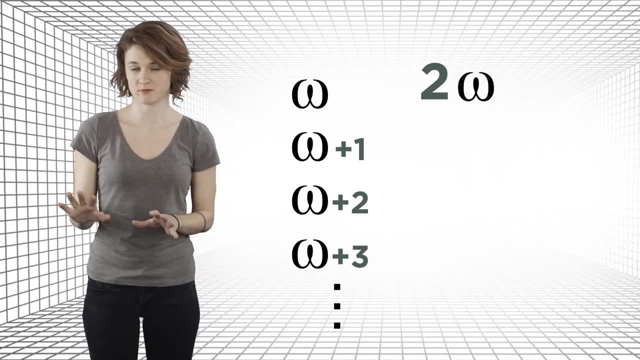 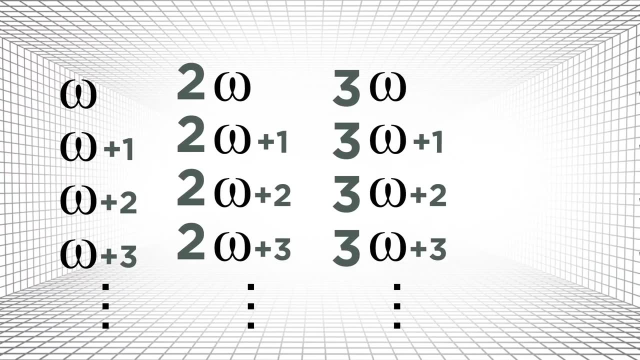 omega plus 3, and so on. Then comes 2 times omega, Then 2 times omega plus 1,, 2 times omega plus 2, and so on. Then there's 3 times omega, 4 times omega, and so on. 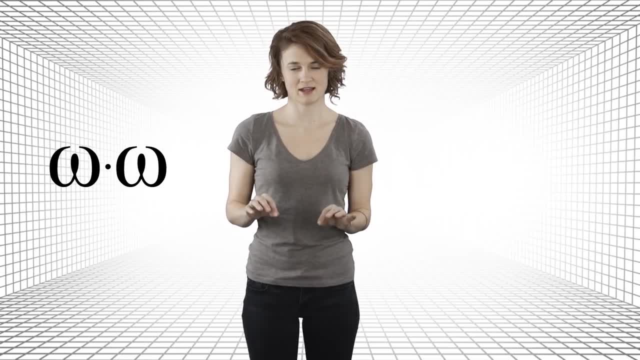 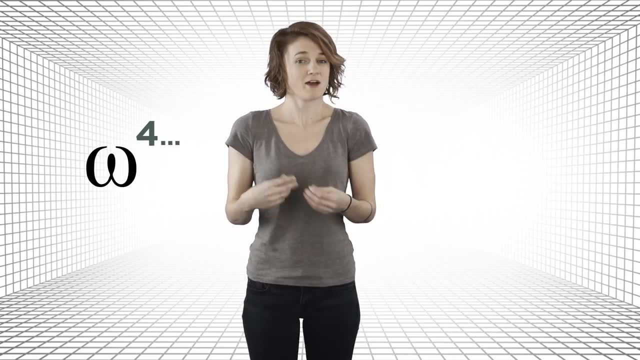 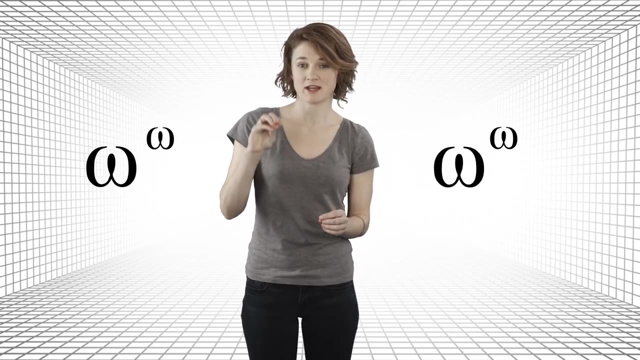 After all that, there's omega times, omega aka omega squared, Then omega cubed, omega to the fourth, and so on. After all that, there's omega to the omega And it kind of just keeps going: Omega to the omega, to the omega, and so on. 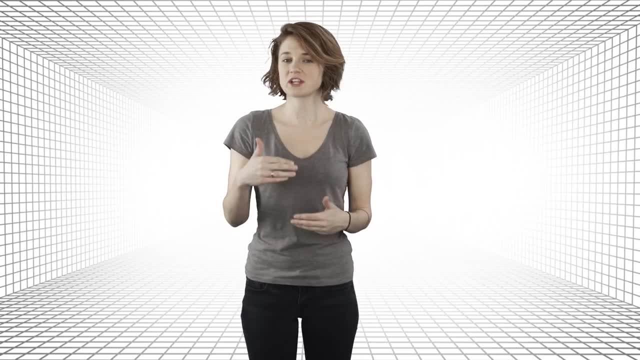 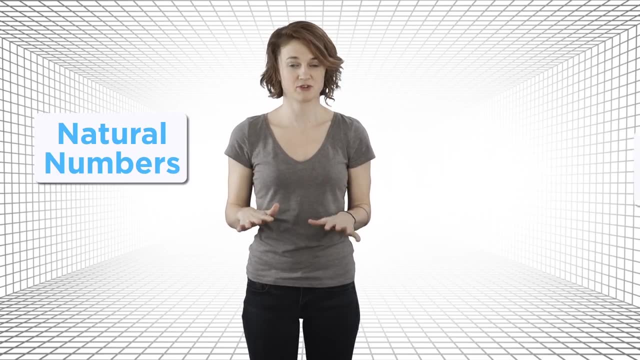 Luckily the ordering is pretty intuitive. You just have to think about the normal order of the natural numbers and then just add a new thing that's bigger than all the natural numbers: omega. So omega to the omega plus 2 is bigger than omega to the 100,. 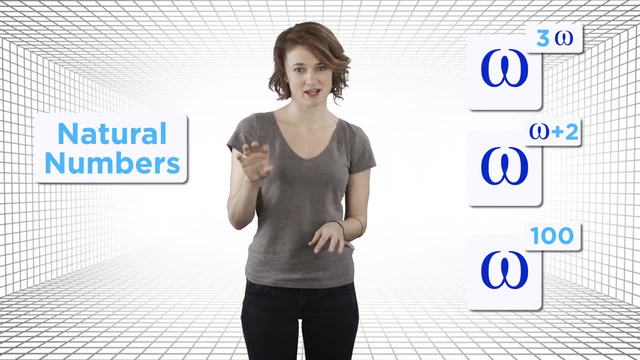 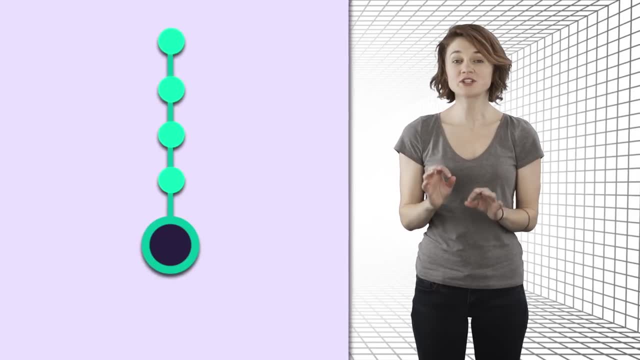 but smaller than omega, to the 3 times omega. Now, how do ordinals help us encode the hydra's complexity? Well, we're going to assign each hydra an ordinal number Each time we chop off a hydra's head. 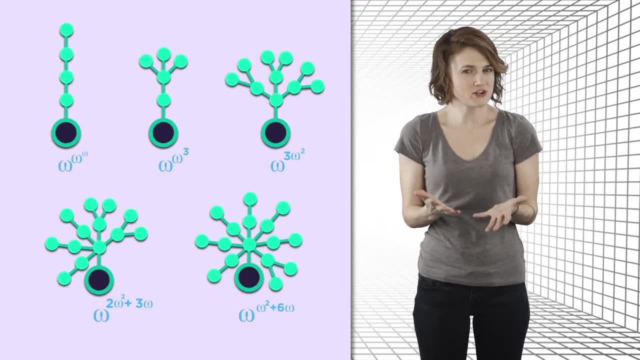 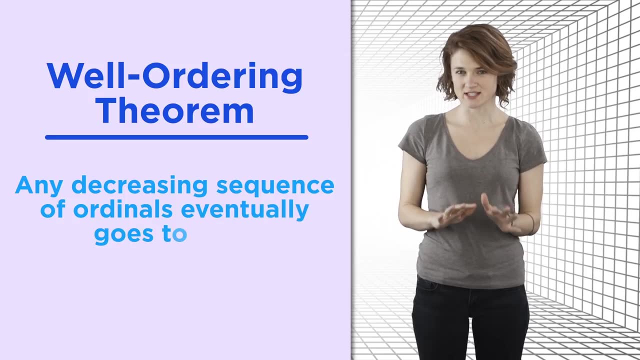 the associated ordinal will decrease. There's a helpful theorem called the well-ordering theorem, which implies that any decreasing sequence of ordinals eventually goes to 0. This means that our hydra will be defeated, no matter what order one chops off the heads. 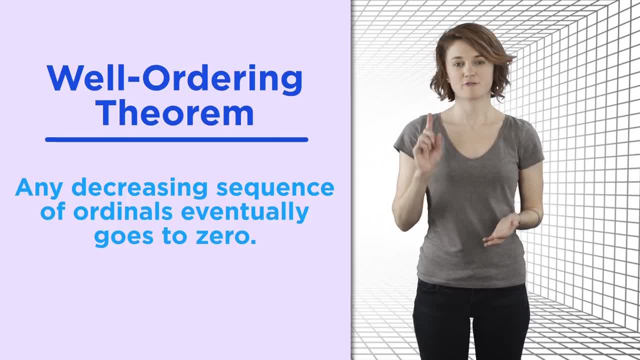 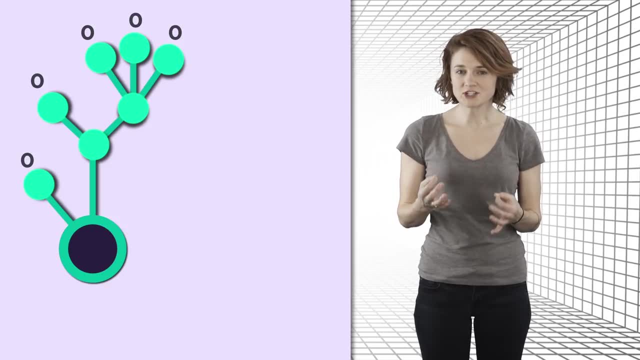 But how do we assign the ordinal to the hydra? 3 times omega squared, 4 times omega squared. First, label all the leaves with a 0. Then, moving down the hydra, we'll label each head according to the ones that are above it. 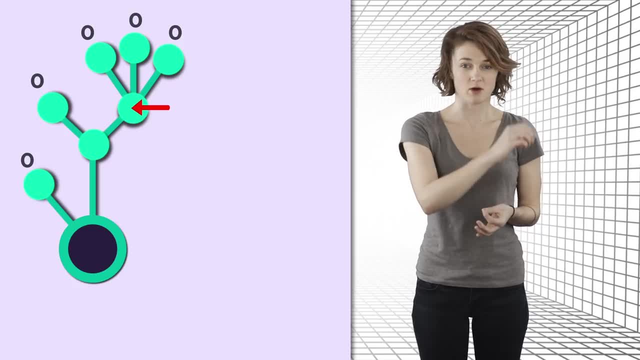 If a head has n heads coming out that are labeled L1, L2, up to Ln, then we label it omega to the L1, plus omega to the L2, up to omega to the Ln. We keep doing this all the way down the tree. 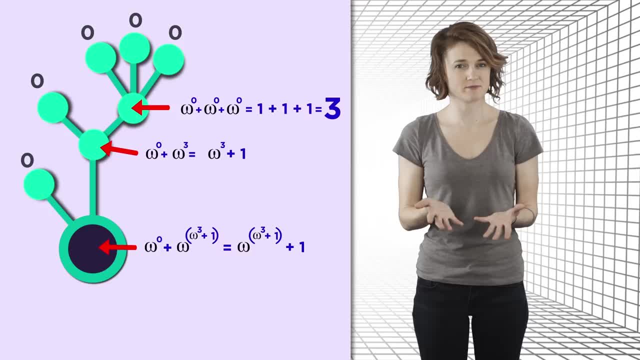 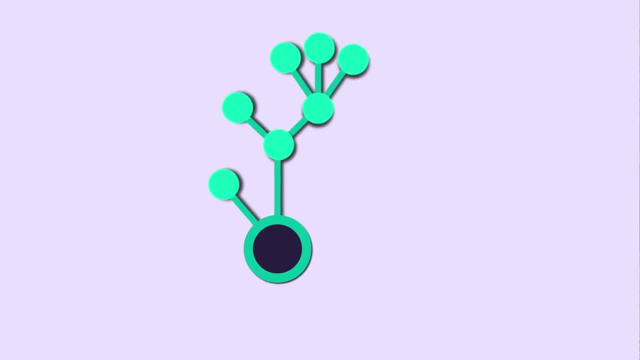 The label on the bottom the body is the important one. It's the ordinal that we assign to the entire hydra. To get the hang of this, let's label this hydra. It's the one that came about when we first. 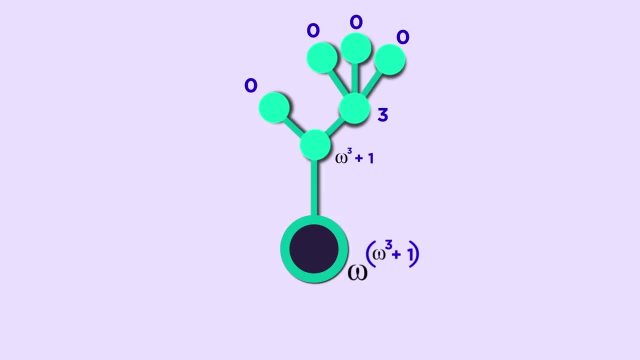 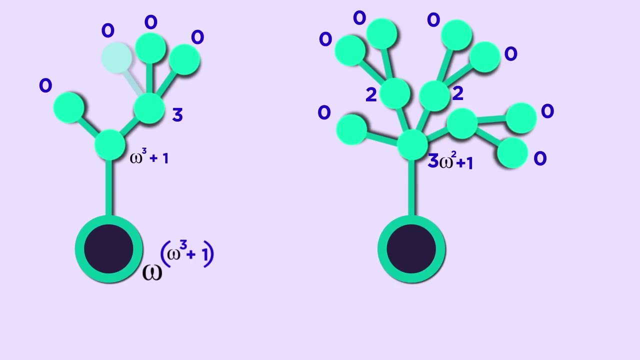 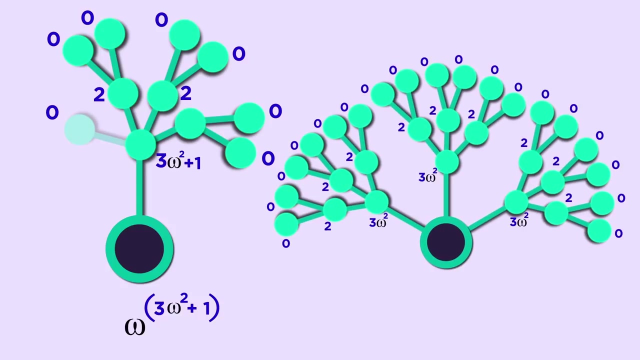 chopped off the lower head- Here's the way we label this hydra- to get its ordinal. Then we chopped off another head and this hydra was the result. Here's the ordinal for that one. Finally, we tried for a third chop and got this hydra. 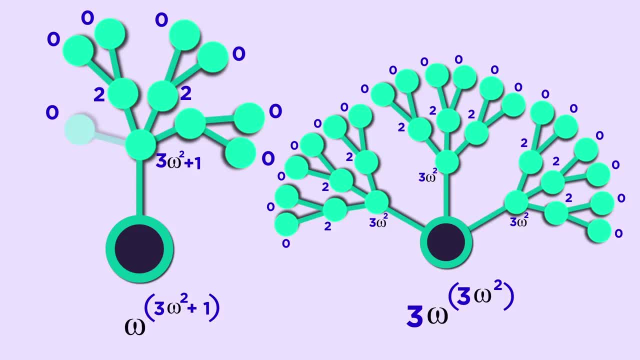 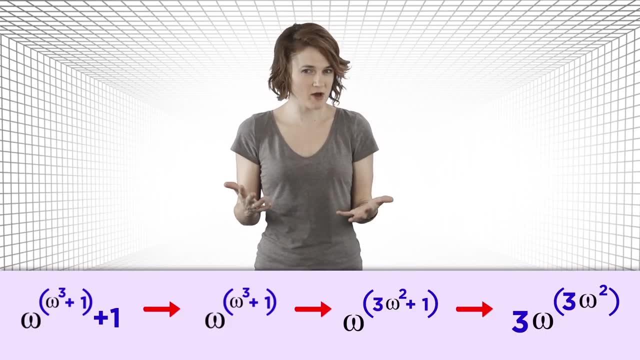 Here's the ordinal. Here's the ordinal for that hydra. Each time we chop a head off a hydra, the associated ordinal gets smaller. It doesn't matter which head we chop off. the new hydra will always have a smaller ordinal. 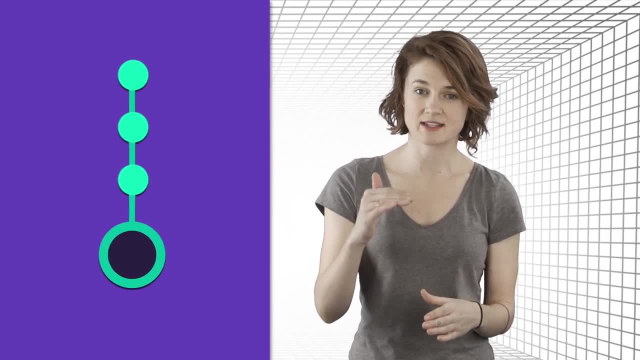 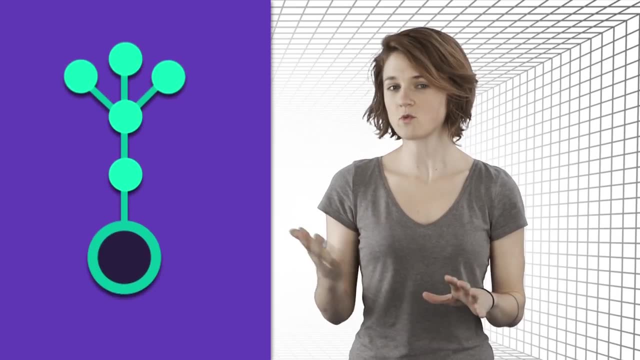 Let's see one more example: the line of three heads stacked on top of each other. The starting hydra has ordinal omega to the omega. After one chop, it's omega. cubed By the sixth step, it's 9.. It's 9 times omega. 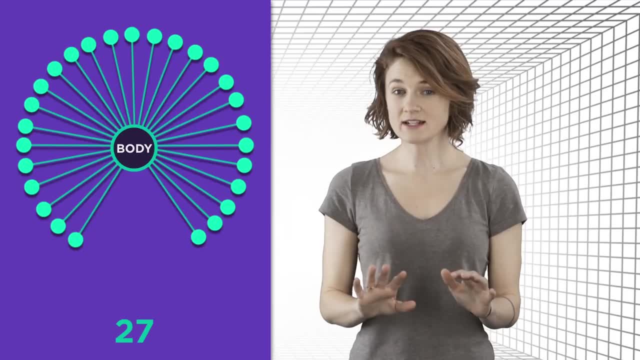 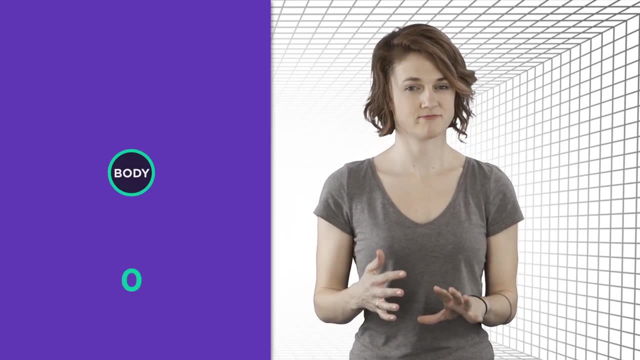 And by the 15th step it's 27.. Finally, after 41 steps, the hydra is just its body. So it is assigned the ordinal 0.. And that's the big point: As we chop off heads the ordinal assigned to the hydra. 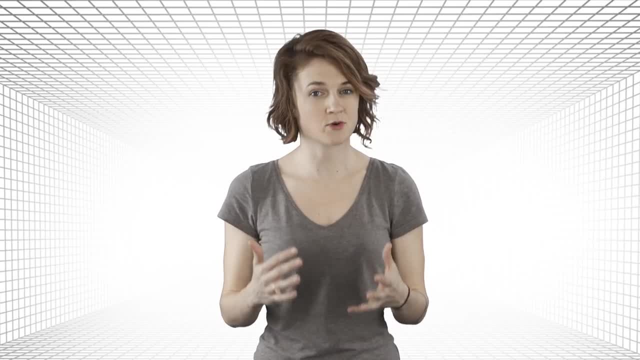 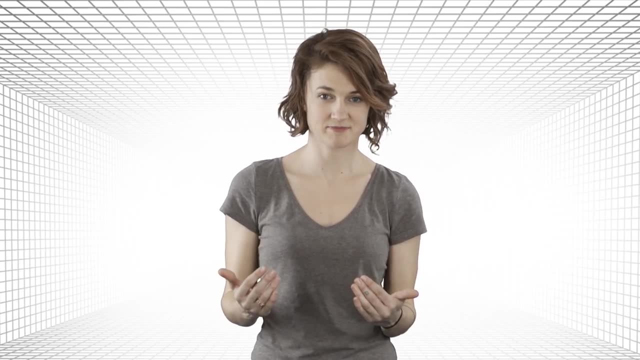 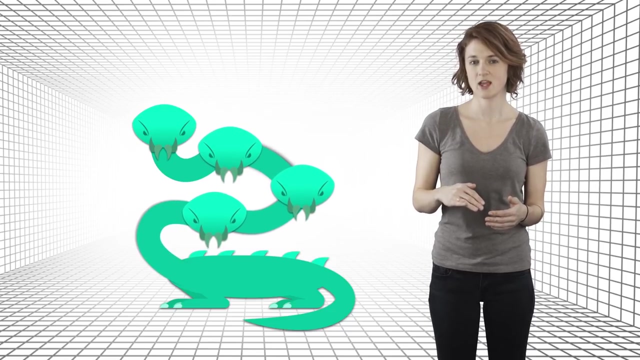 keeps getting smaller and smaller until the assigned ordinal is 0. And when it's 0, that means the hydra has been defeated. It's just a body. The hydra we just defeated grows. two new copies of the part below the chopped off head. 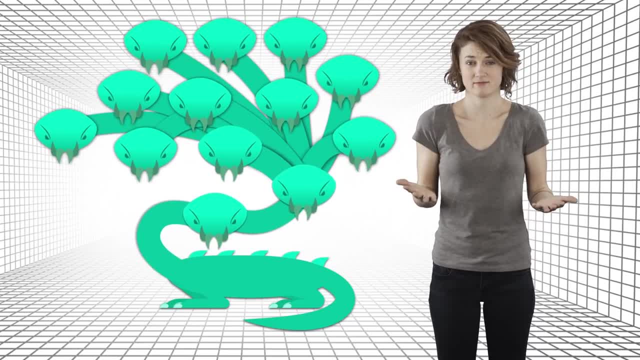 What if it grew three new copies, Or four, Or 10?? Amazingly, not much changes. It's still true that, no matter what order you chop off the hydra's heads, you'll still defeat it in a finite number of moves. 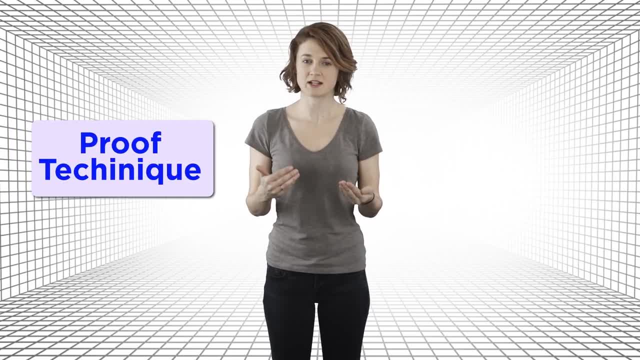 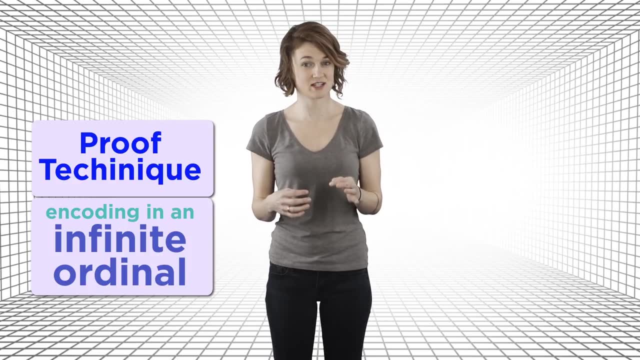 No matter how many heads grow each time, the proof technique that involved encoding the hydra in an infinite ordinal will still be true. The ordinal still shows that the hydra will be defeated. The ordinals will still be decreasing and therefore must eventually be 0.. But here's the part that totally blows my mind. Let's say, the hydra grows. one copy after the first chop, two copies after the second chop, 10 copies after the 10th chop, and so on. With each chop it's regenerating faster. 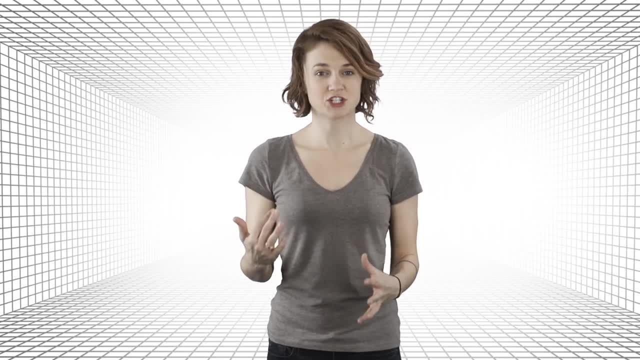 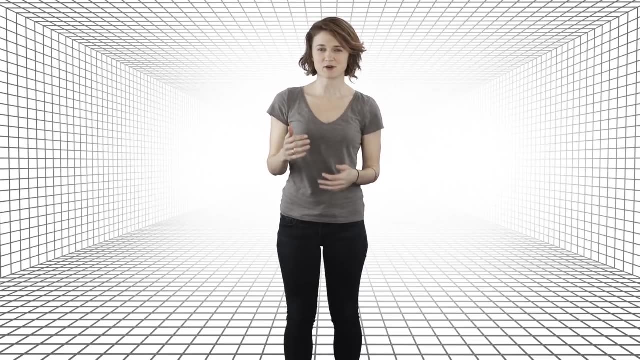 Still, even, still. you'll eventually chop off all the hydra's heads, And the same proof technique shows it. There's a really crazy story behind this hydra: how and why mathematicians developed it and why the proof is so unexpected. 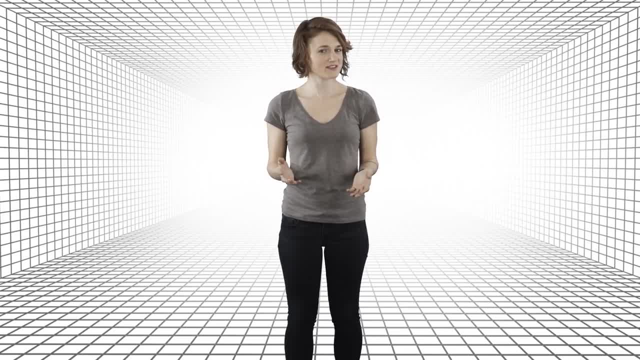 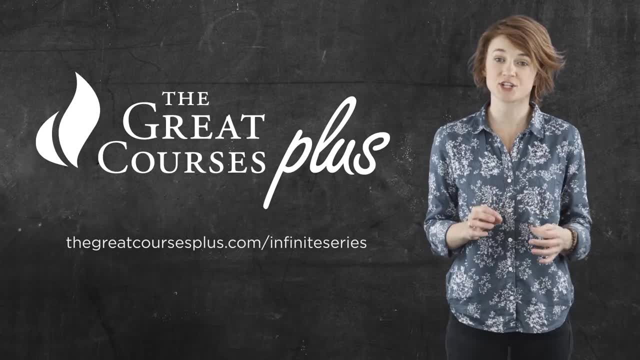 We'll explore this in next week's episode, the prequel to our Slay the Hydra adventure. Thanks to The Great Courses Plus for sponsoring this episode. The Great Courses Plus is a digital learning service that allows you to learn about a range of topics. 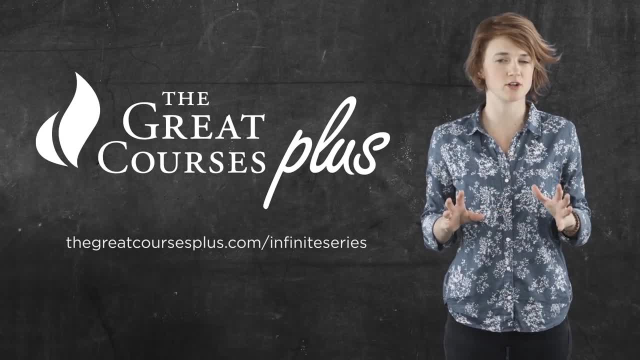 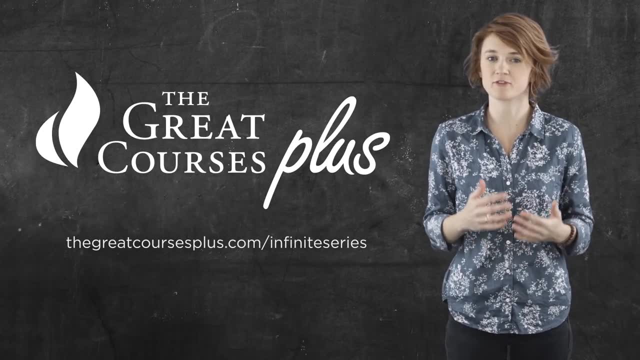 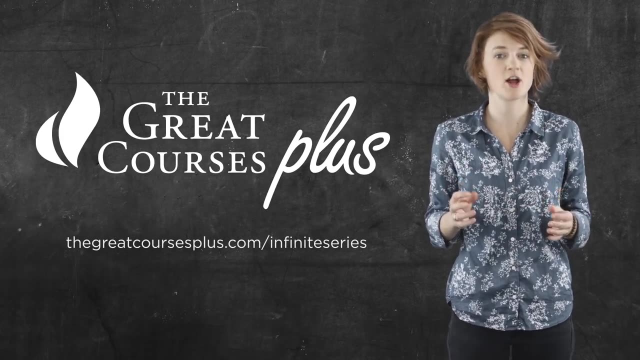 from renowned professors and other educators from all over the world. Go to thegreatcoursespluscom, slash infinite series and get access to a library of different video lectures about science, math, history, literature and even how to cook, play chess or become a photographer. 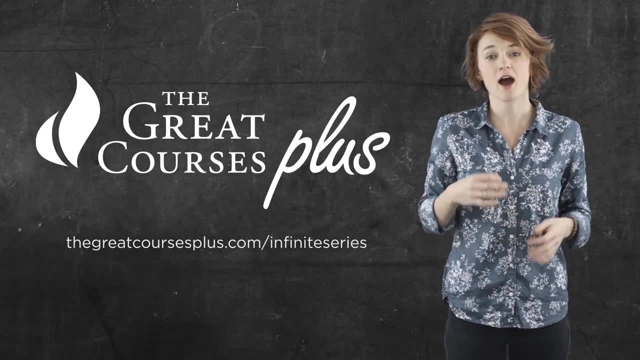 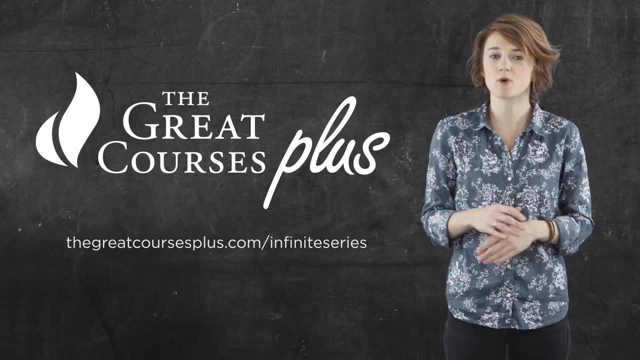 New subjects, lectures and professors are added every month. I'm currently enjoying David Kung's engaging course How Music and Mathematics Relate With The Great Courses. Plus, you can watch as many different lectures as you want, anytime, anywhere, without tests or exams.